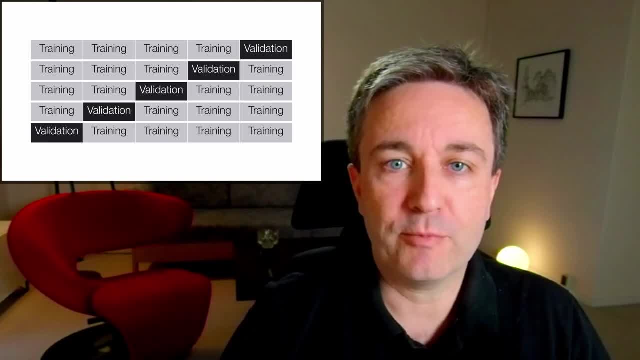 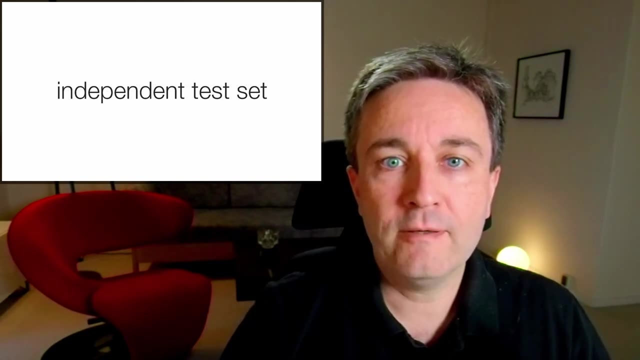 That is, you split, for example, your data into five different partitions and, in a round-robin fashion, use all the data to validate the models predicted on the other parts of the data. Regardless of whether you have a single validation set or you do cross-validation, you need an 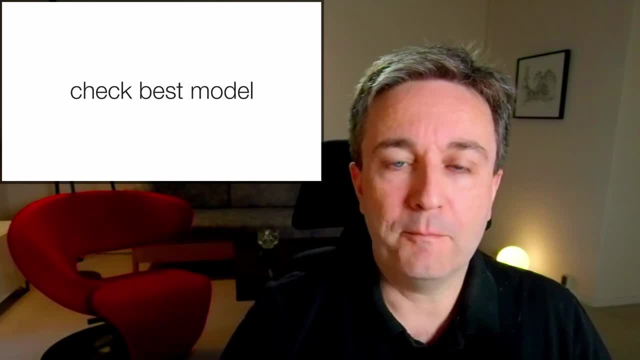 attempt set. This set is used to check the best model that you've selected based on the validation set, and to ensure that you have no overfitting and thus get the final performance estimates. that should tell you how well the model will generalize to new examples. 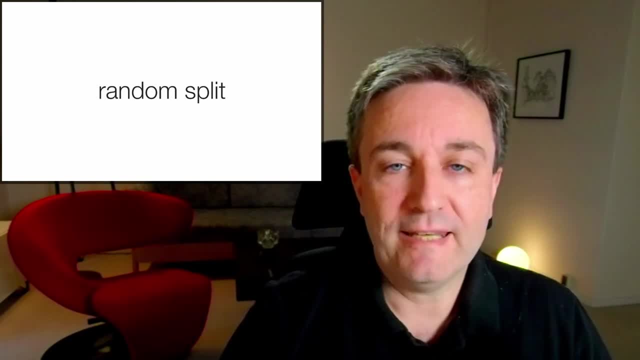 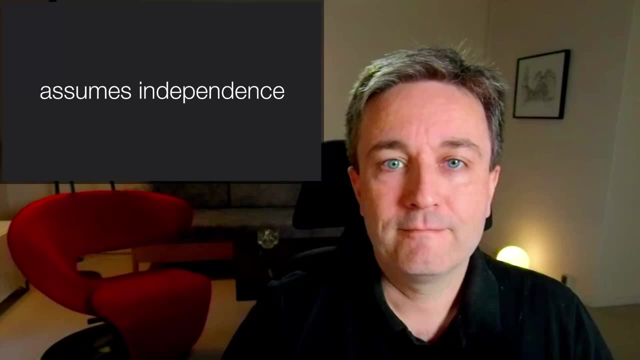 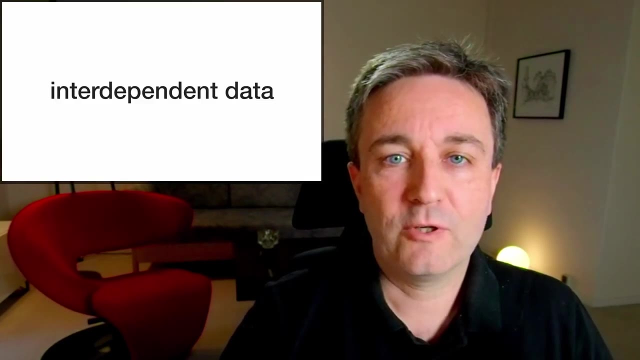 When you make these different data sets- training, validation and test- it's typically done by doing a random split or partitioning of the examples. The problem here is that this approach assumes independence between the different examples. Unfortunately, interdependent data are common in biomedicine and that is a big problem when 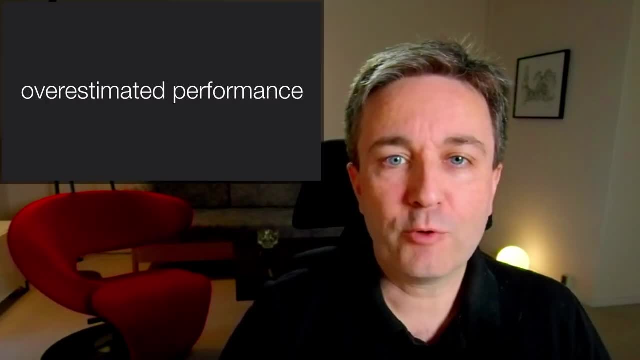 you want to apply machine learning in this domain. The problem is that it leads to overestimated performance and thus to publication of bad methods that quite simply do not work anywhere near as well as claimed in the papers. To understand this, let's think about some examples. 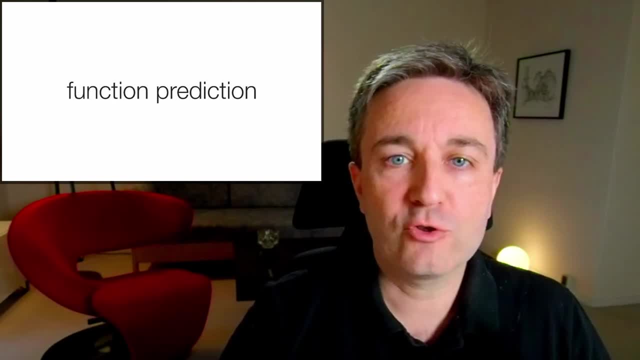 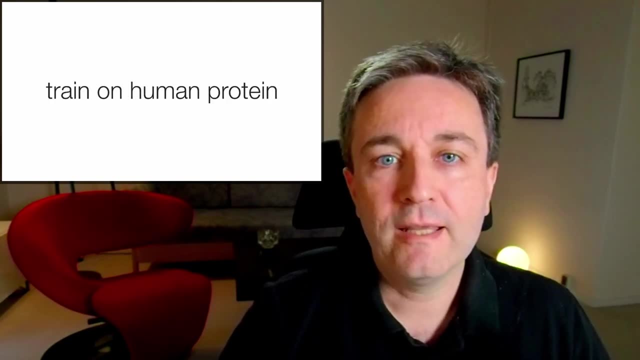 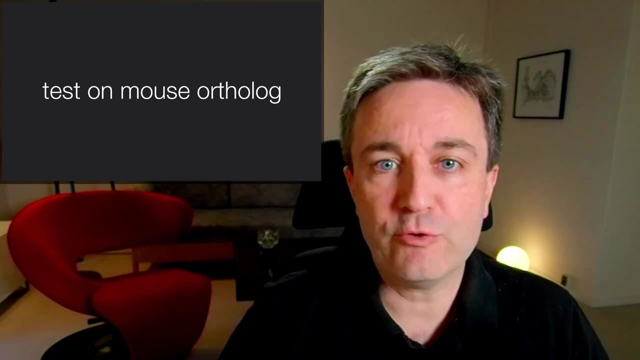 In sequence analysis. you might want to train machine learning to predict function. In this case you need to worry about common ancestry in your data set. For example, it would not be okay to train on a human protein and then test the performance on the mouse-author log of the same protein. 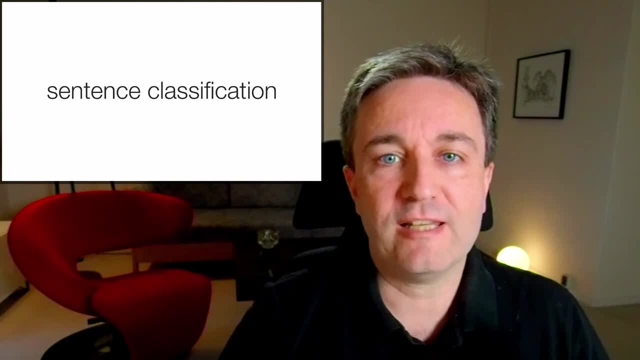 Similarly in text mining, you may want to do sentence classification, in which case you should worry about common source of the sentences. That is, it would not be a very a good idea to train on one sentence and test on the very next sentence from the same paper. 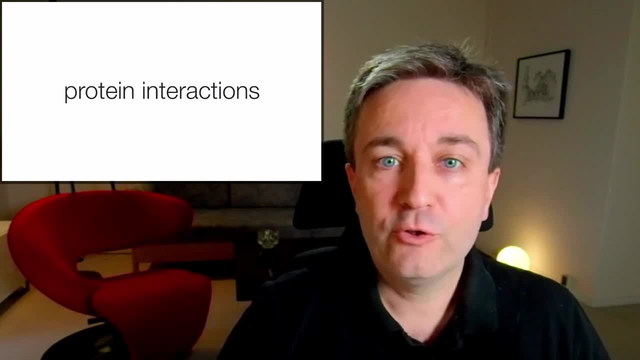 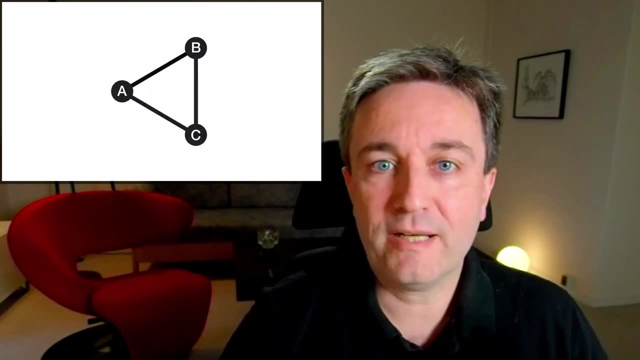 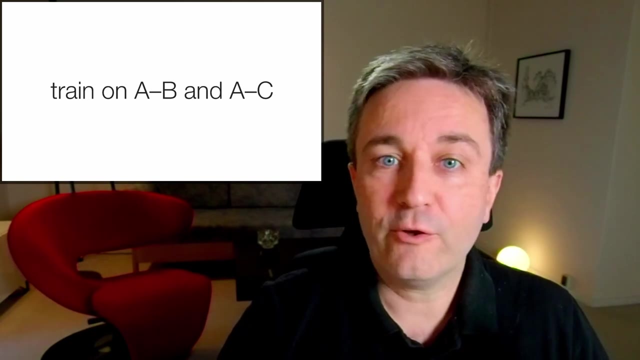 If you're working on protein interaction networks, like I do, you need to worry about common nodes in your network. That is, when you have an interaction network of a complex ABC, it will be represented as this binary network. In this case, you cannot train on the interactions AB and AC and then go.